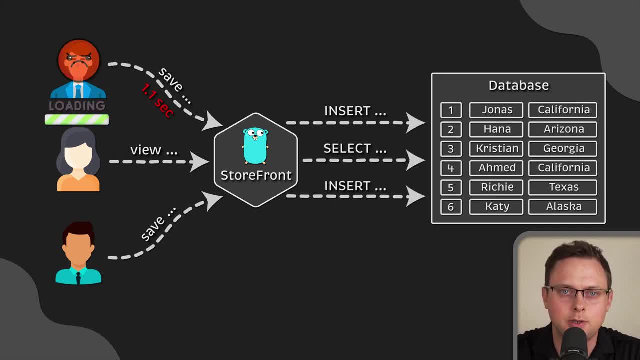 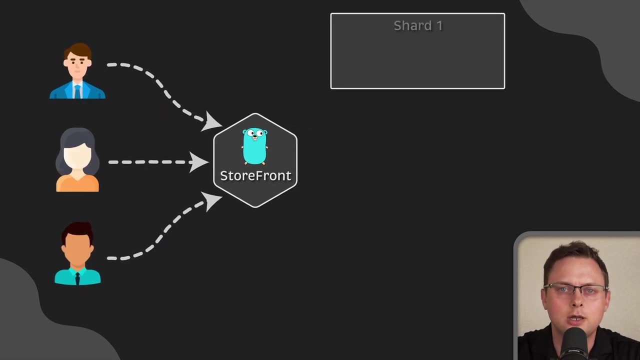 increases over the time. Now the database becomes a bottleneck. if too many users attempt to use the application to read or save data simultaneously, The application slows down, negatively affecting the user experience. So sharding not only allows you to store more data, but also improves. 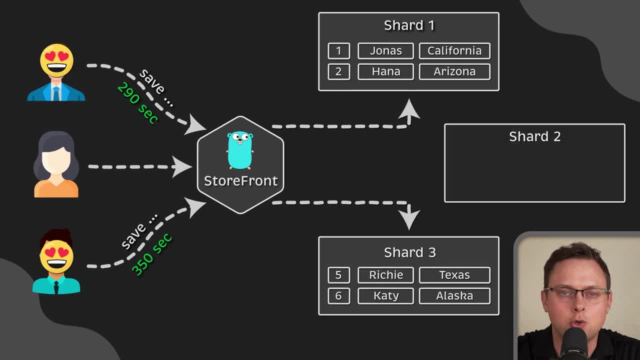 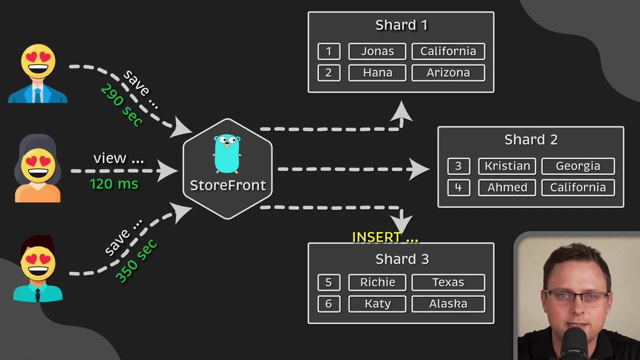 performance by reducing latency for each query. This is because you can now push down the query to each individual shard, So you can now push down the query to each individual shard which has a smaller dataset. There are three main reasons why you should be using sharding. 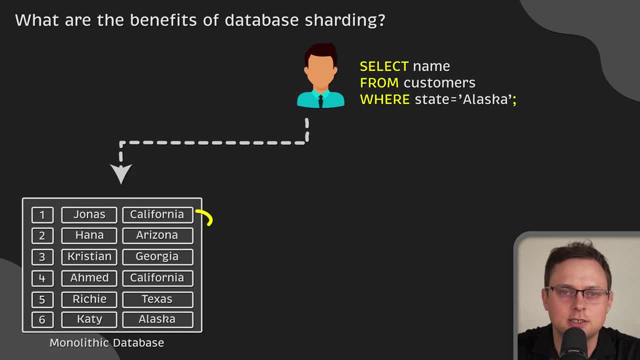 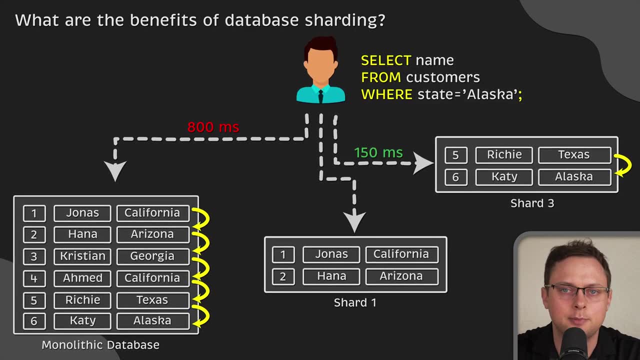 First of all, response time. By splitting a database into smaller datasets, it improves query performance, as it needs to search through fewer rows compared to a monolithic database. Second, it can help to avoid total service outage Most of the time. 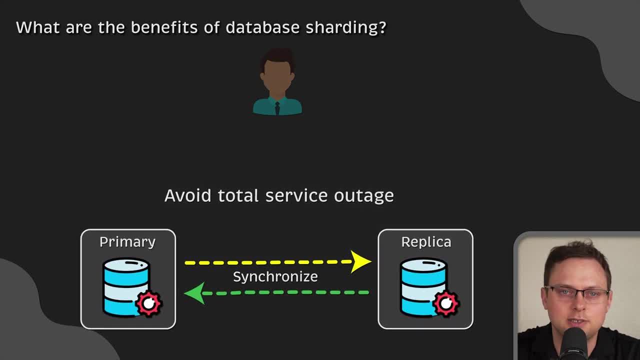 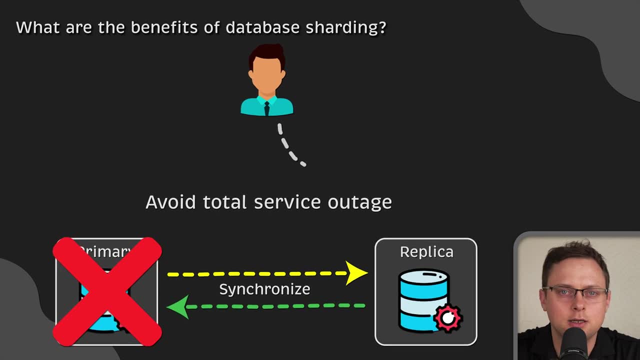 we're not only splitting data across different database servers, but we also configure replication. So if you want to use sharding, you need to use sharding. So if one shard becomes unavailable, the data can be accessed and restored from another shard. 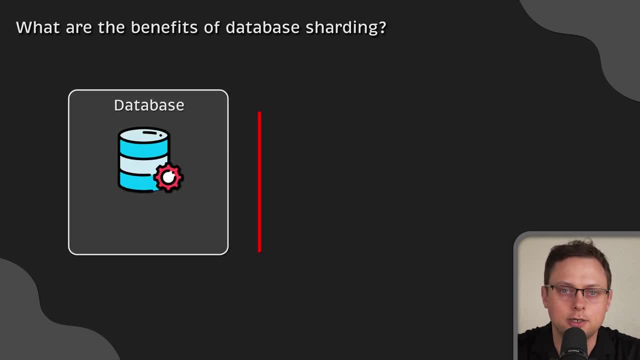 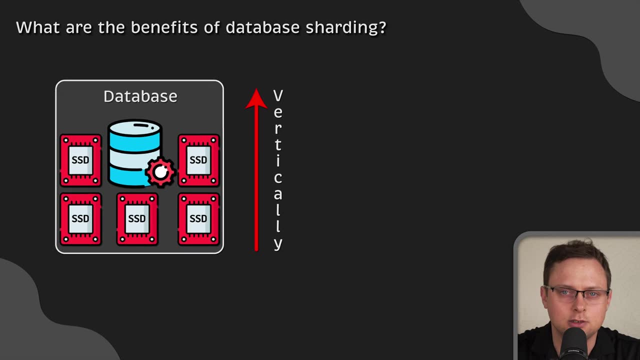 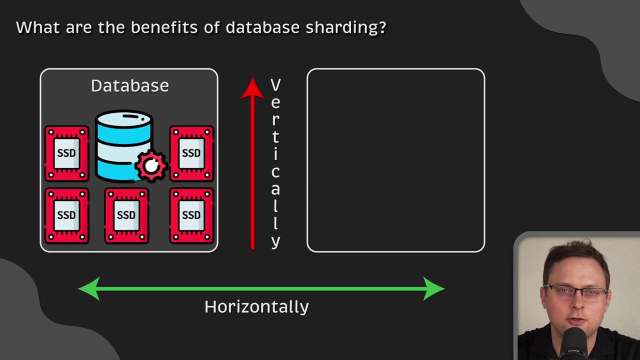 Finally, a growing database consumes more computing resources and eventually reaches storage capacity. There are only so many disks you can attach to a single server. Therefore, sharding can solve this problem by scaling the database horizontally instead of vertically. Also, you can add shards at runtime without shutting down. 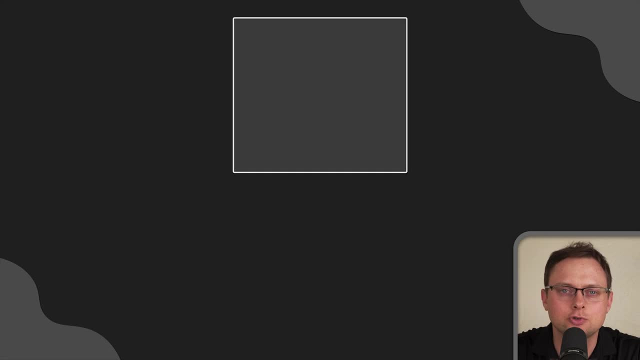 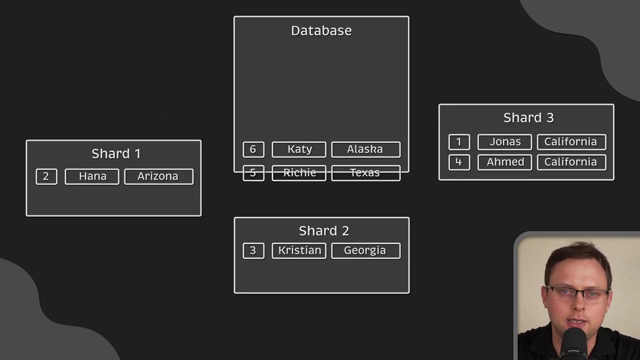 an application for maintenance. Now let's see how sharding works. A typical unsharded database stores data in multiple columns and rows, So database sharding splits a single dataset into partitions or shards. Each shard contains unique rows of data which are stored separately across multiple computers. 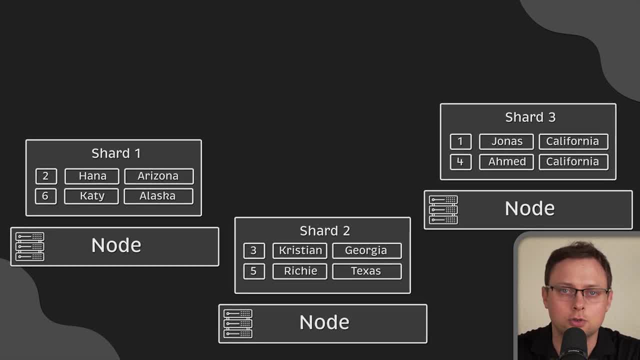 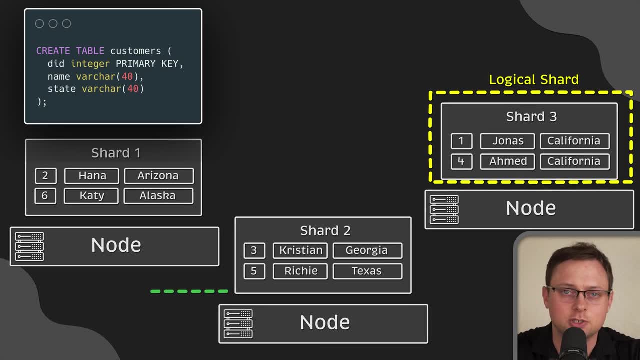 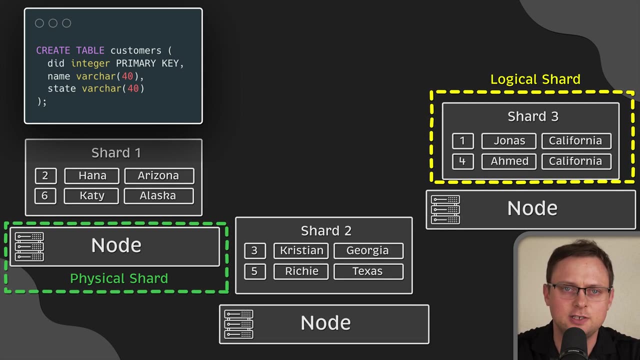 called nodes. All the shards run on separate nodes but share the same schema or design. The partitioned data chunks are called logical shards. The machine that stores the logical shard is called a physical shard or database node. Keep in mind that a physical shard can contain multiple logical shards that belong to the same table. 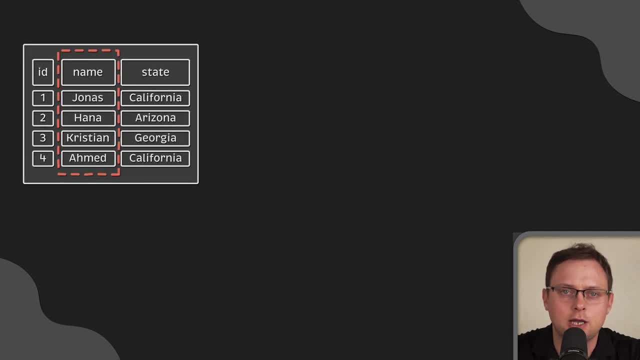 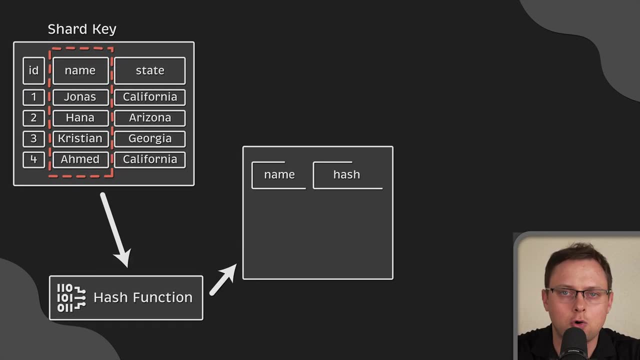 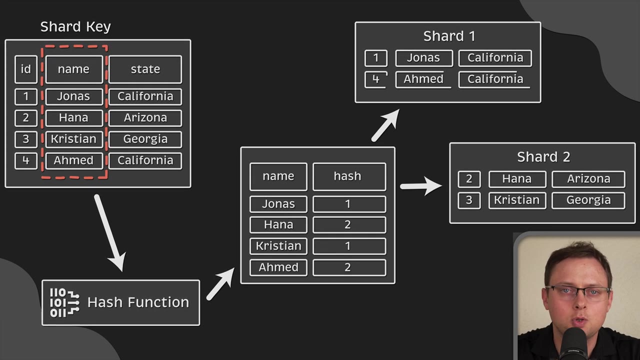 Now software developers would use a shard key to decide how to partition a dataset. A column in a dataset, such as customer name, determines which rows of data group together form a shard. Developers can choose a shard key from an existing column or create a new one. 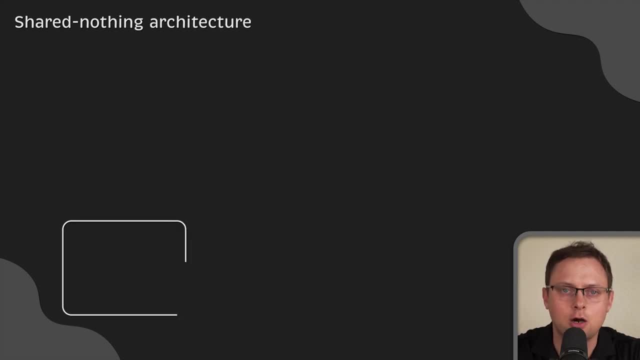 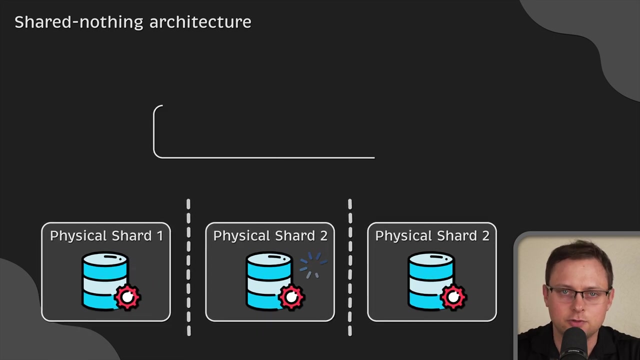 Database sharding operates on shared-nothing architecture. Each physical shard operates independently and is unaware of other shards. Only the physical shards containing the data you request will process that data. in parallel, Above the shard, we have another abstraction software layer that coordinates data storage and data storage. 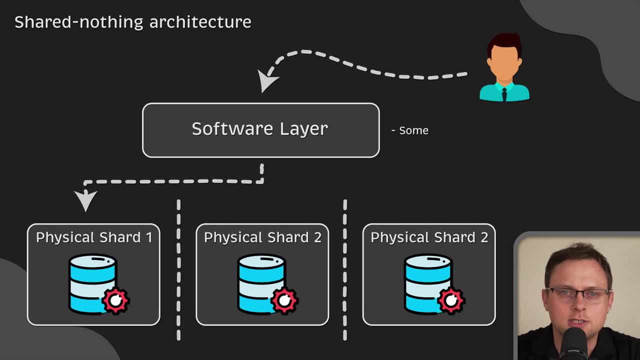 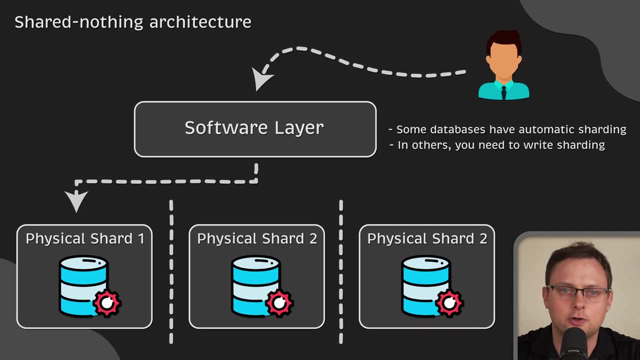 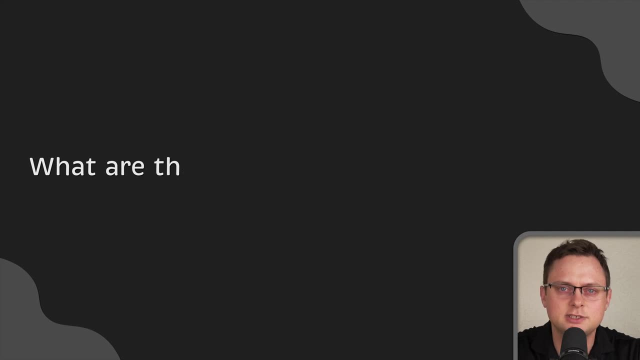 Sharding can be used to store or retrieve data from multiple shards. For instance, some databases have automatic sharding features built-in. In others, you, as a software developer, need to write sharding code to store or retrieve data from the correct shard. Now let's discuss different. 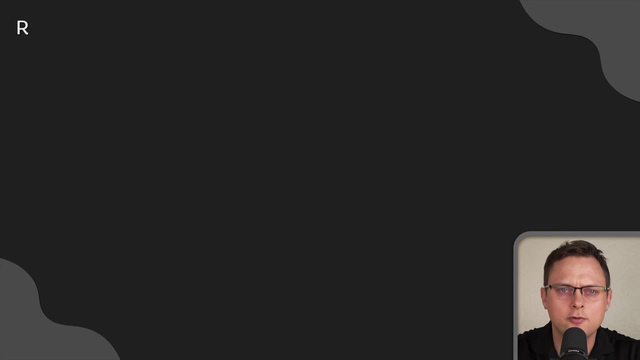 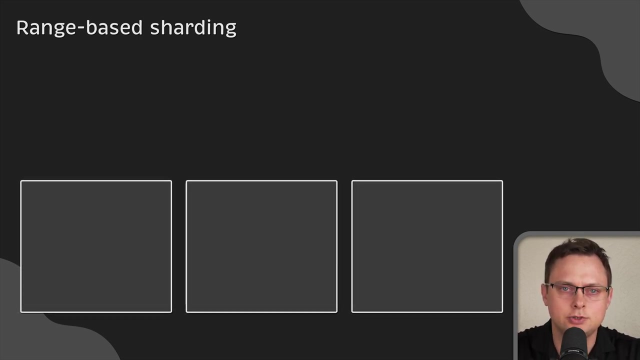 approaches you can take to shard your database. One of the simplest methods might be to use range-based sharding, also known as dynamic sharding. This approach splits database rows based on the range of values. For example, suppose you decide to use customer's name as a sharding key. Now let's say you want to create three shards. 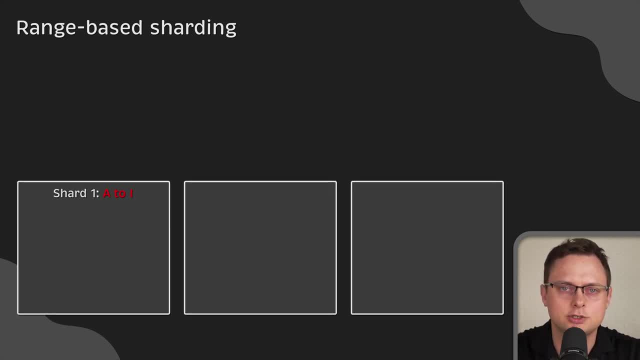 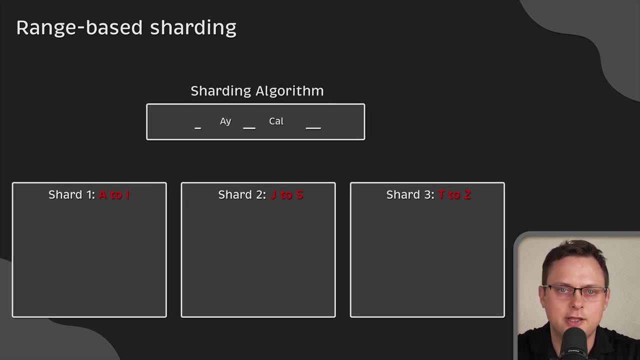 In the first shard you would place all customer records if the customer's name starts with a letter between A and I. For the second shard, you would use letters J through S And for the third one you would use T through Z. Every time you write or retrieve. 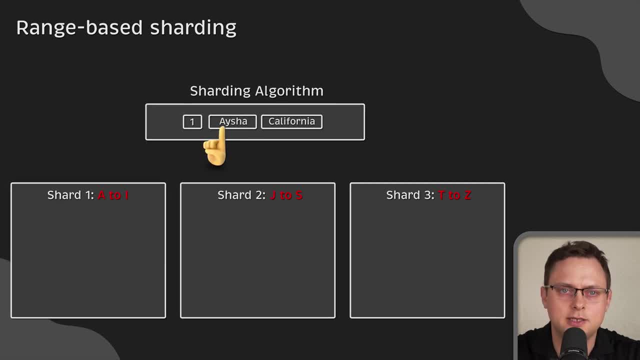 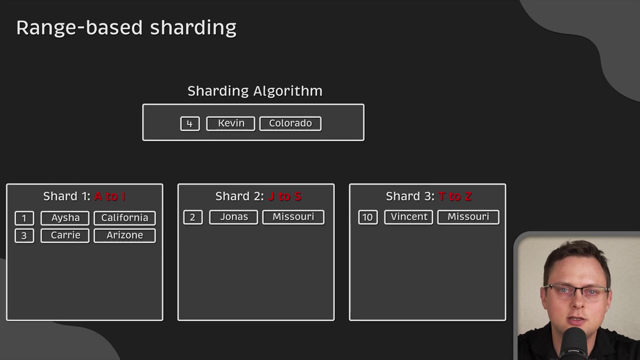 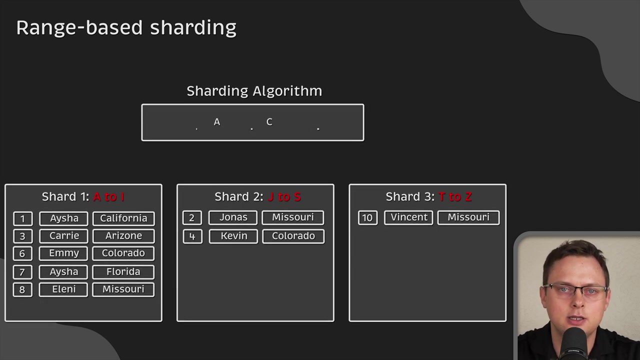 data from the database. your application or database checks the first letter of the customer's name and places that record in the corresponding shard. Depending on the data values, range-based sharding can result in overloading of data on a single physical node. In our example, the first range from A to I might contain significantly more customer names. 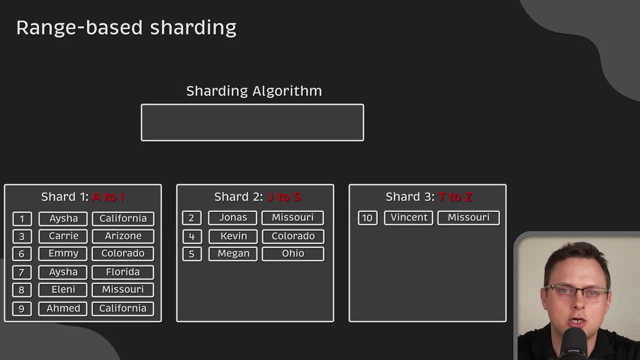 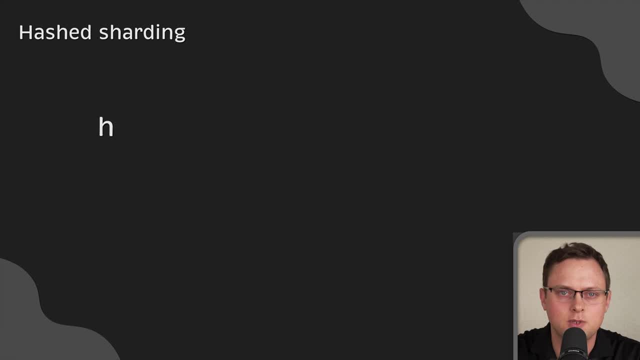 than, for instance, the third shard, where names with T to Z. However, this method is easier to implement. The next method is hashed sharding. In this case, we use a mathematical formula and apply it to each row in the database. For example: 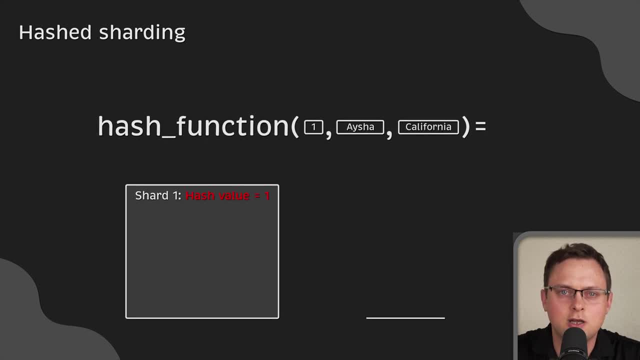 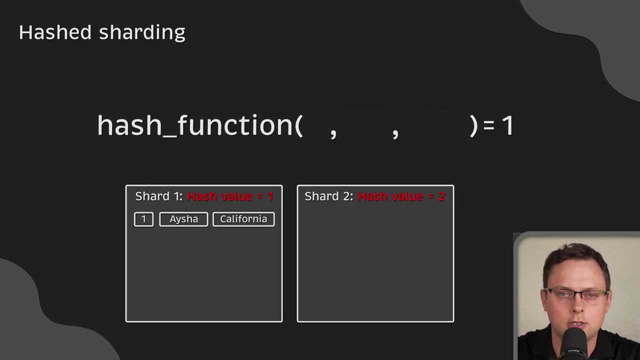 in this case we can have two shards. So if the hash function takes all the customer record values and produces one, we will store it in shard number one, And if the hash function returns two, we will store it in the shard two. 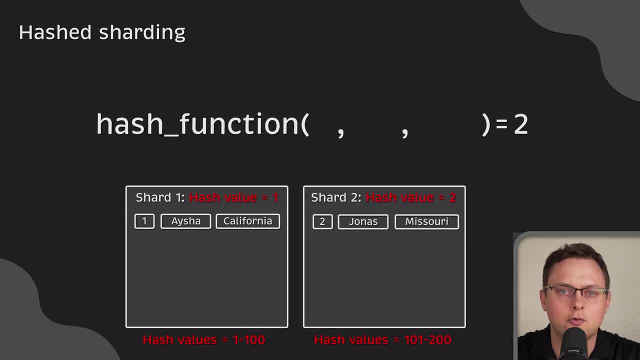 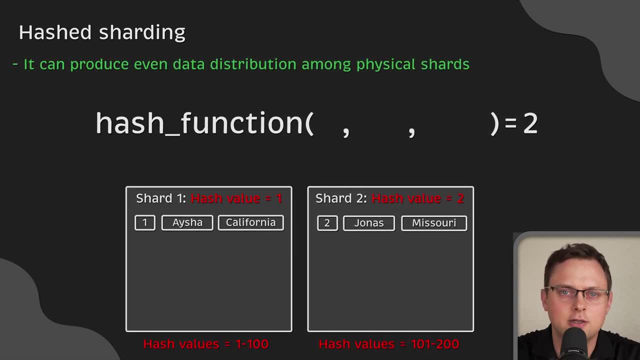 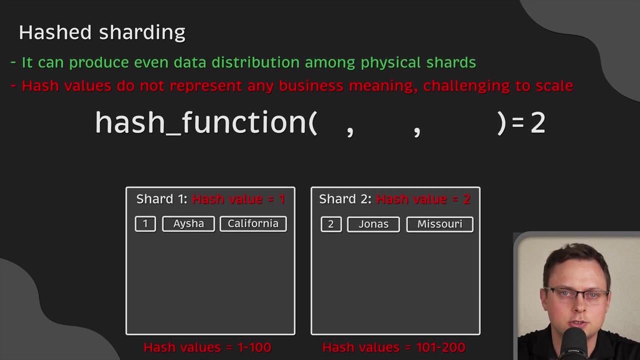 In the real world. these shards, of course, operate on a range of hash values that the function can return. The benefit of this approach is that it can produce even data distribution among physical shards, But, on the other hand, since these hash values do not represent any, 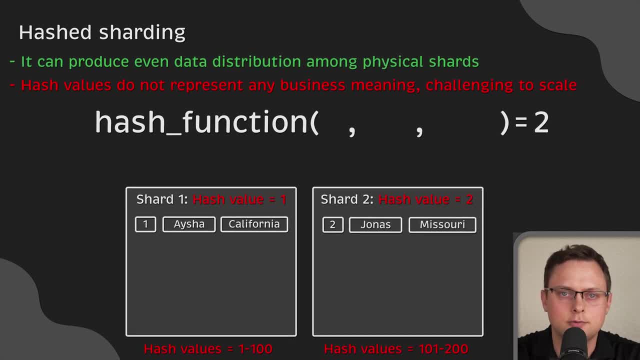 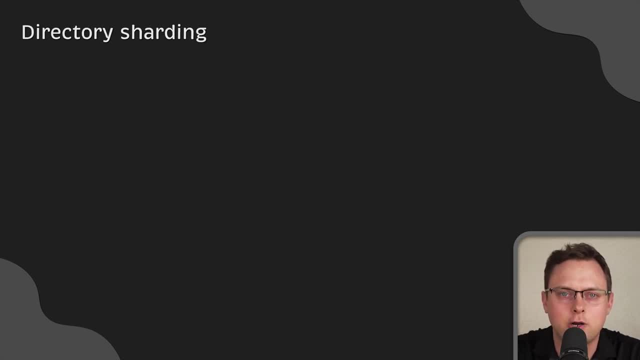 business, meaning it may become challenging in the long run to reassign the hash values when adding more physical shards. Another way you can use is directory sharding. This approach uses a lookup table to decide where to store the record. For example, let's consider that you may store some items in the database. 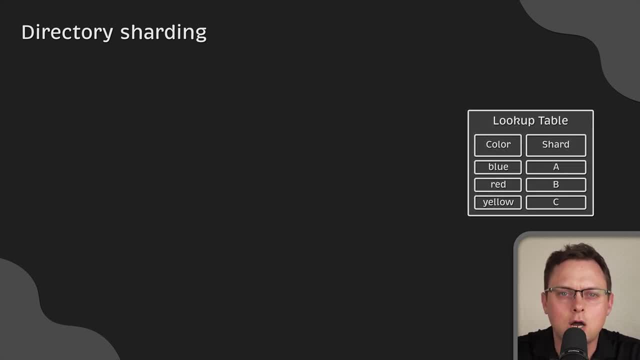 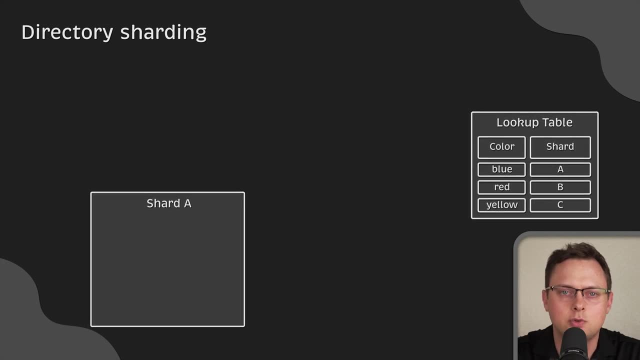 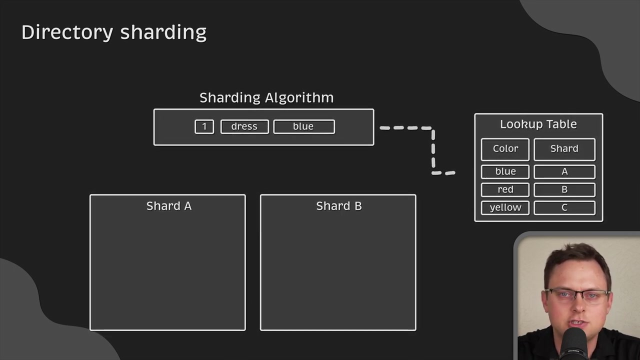 and you can have item color lookup table. Each color would have its own shard. For instance, blue items will be stored in shard A, red items will be stored in shard B, etc. This approach is very flexible. Each shard is a meaningful representation of the database. 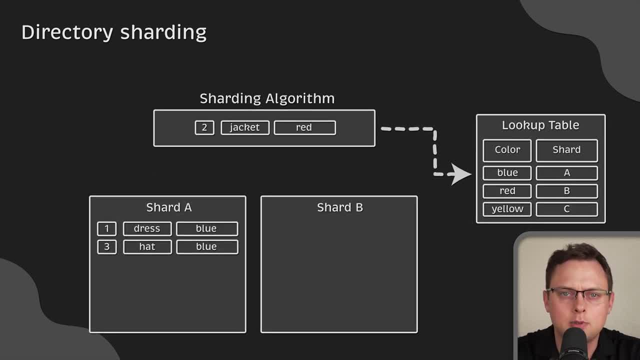 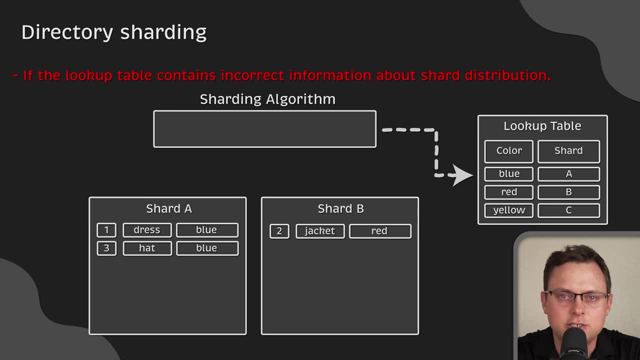 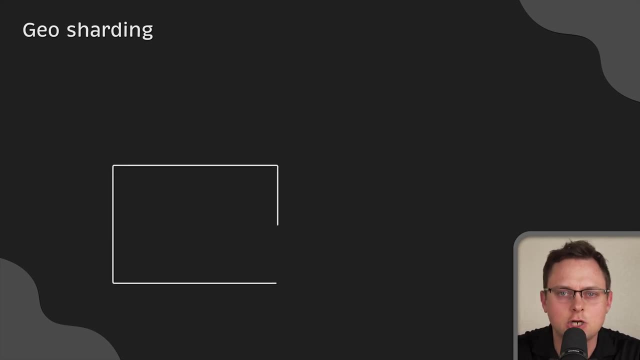 And it is not limited by ranges. The only problem you may face is if something happens to your lookup table And if the table contains incorrect information about shard distribution. The last type that we are going to discuss is geosharding. This type of sharding is based on: 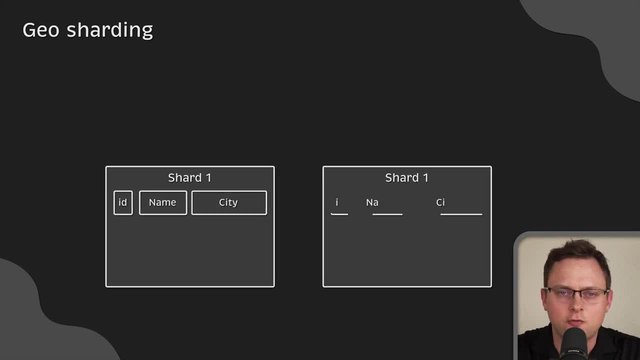 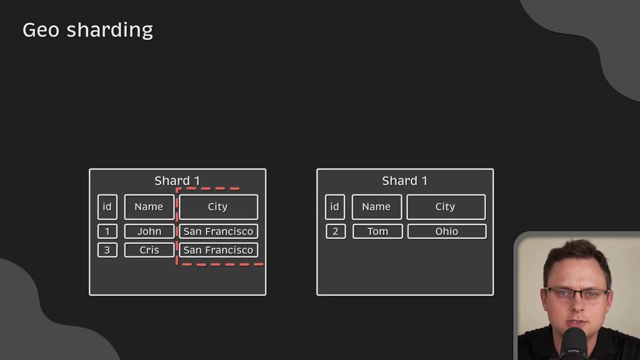 the physical geolocation associated with the record. For example, a dating site can store users in different shards based on their locations. You can use the city as a sharding key to decide where to place the record. The biggest advantage of this approach: 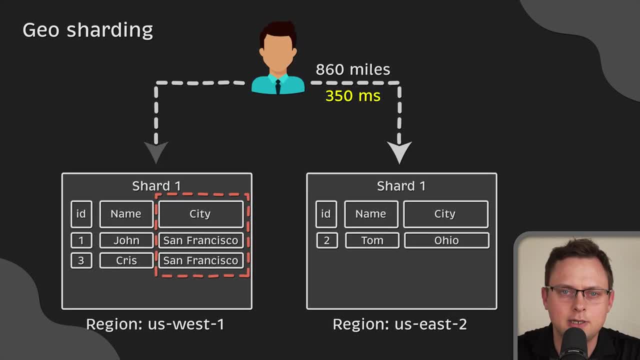 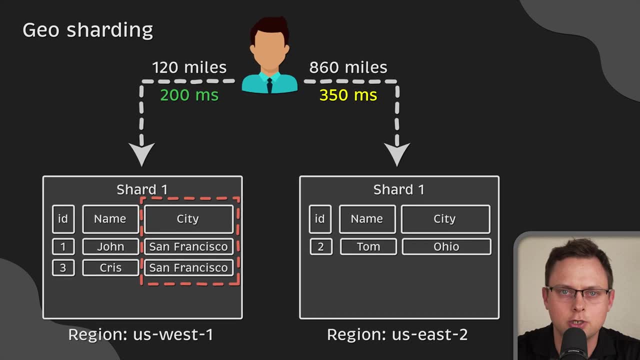 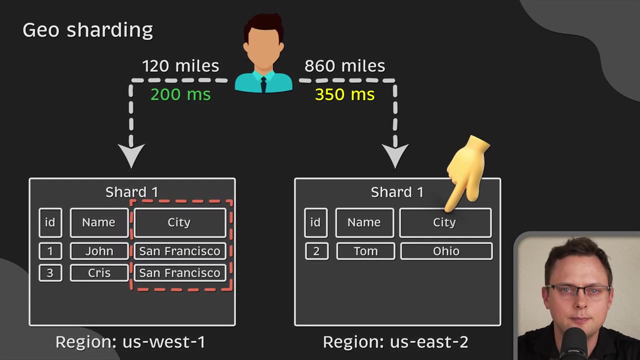 is that you can now serve relevant data from the database in the same region. Therefore, since the distance between the end user and the data location is shorter, the response time will be also improved If the data access patterns are mostly based on geolocation, this approach 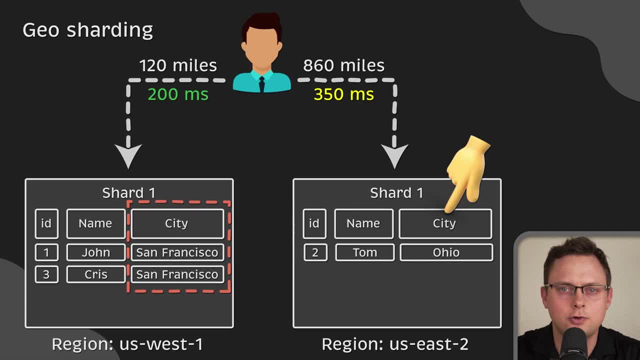 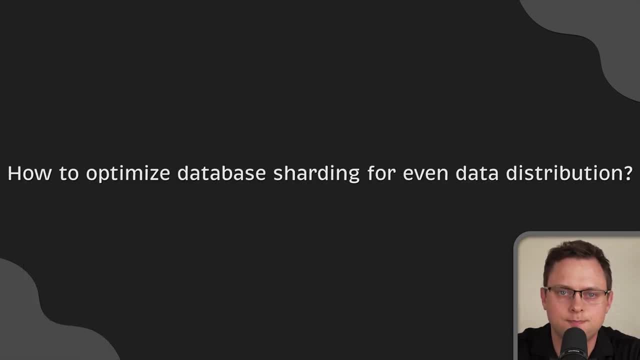 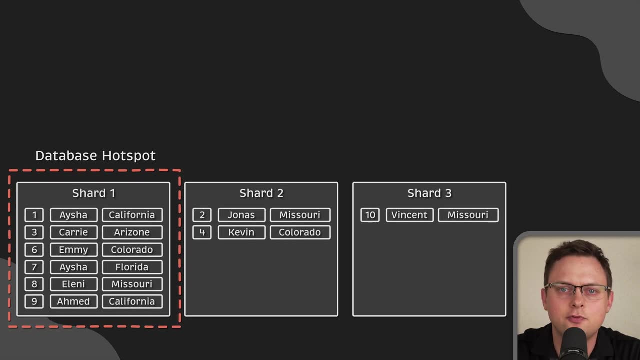 works great. However, geosharding can also result in uneven data distribution. Now let's talk about how to properly select a sharding key. When a data overload happens on the specific physical shards and others remain underloaded, it results in database hotspots.